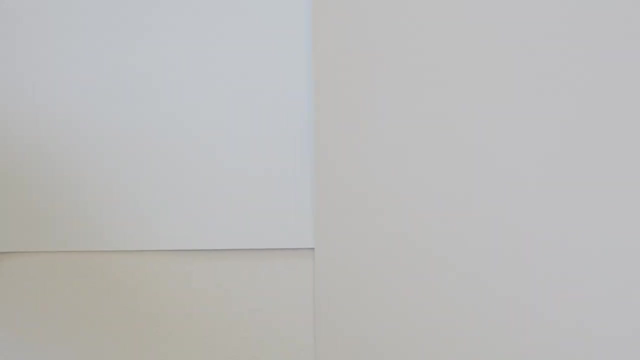 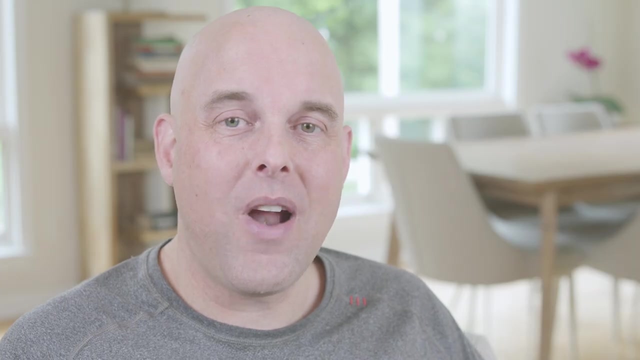 is. I'm going to show you the difference between a cool gray and a warm gray, And then I'm going to show you four different undertones that you need to know about cool blue grays and why this is important. And then I'm going to show you two different undertones of warm. 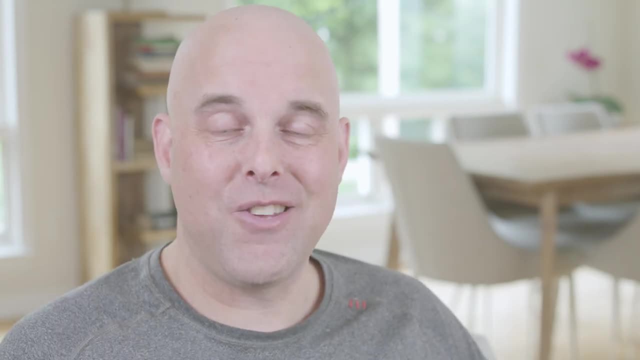 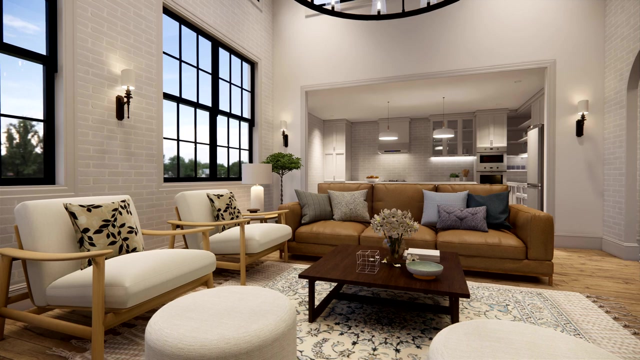 grays and why you need to get this right, And then, towards the end of this video, I'm going to talk about why the fixed elements and lighting will play a key role on how each one of these paint colors could look like in your home. And for those of you that don't, 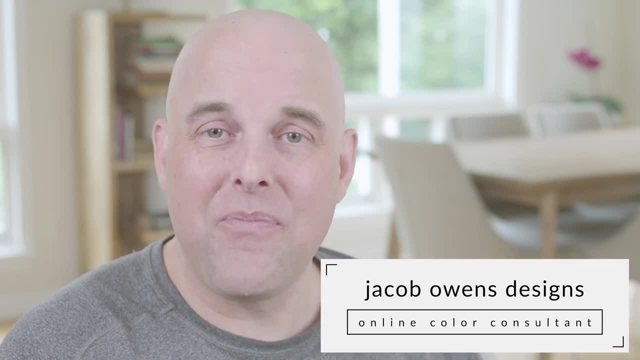 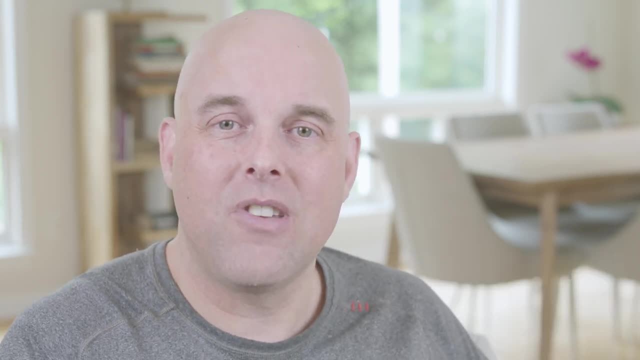 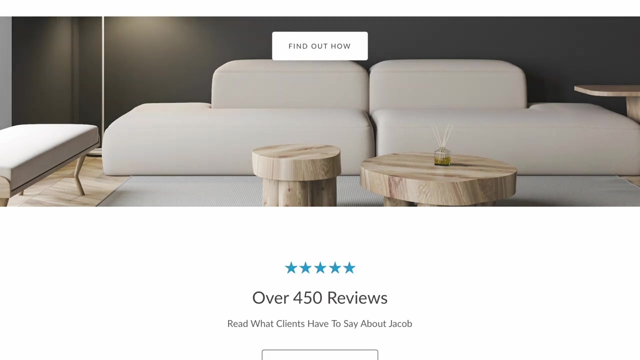 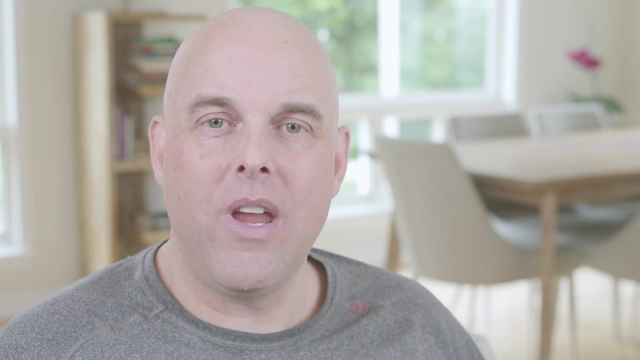 know who I am. I'm an online color consultant. I help thousands of clients all over North America select the perfect interior or exterior paint color for their home, And I'm going to show you the difference between a cool gray and a warm gray. So the first thing, 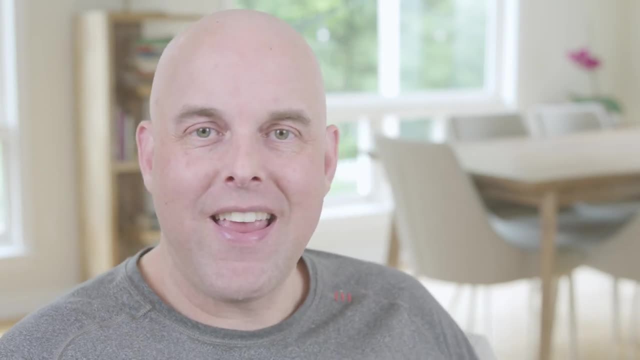 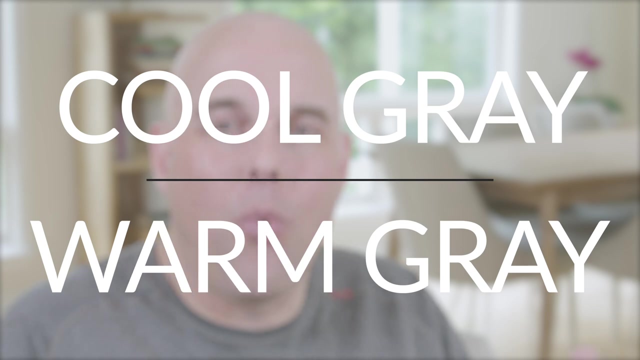 I want you to know about gray paint colors is. there's no such thing as a perfect, neutral gray paint color. It doesn't exist. It's really simple. There's either a cool gray or warm gray. That's it, And the best way to explain it is to show you. So I'm going to use Stonington. 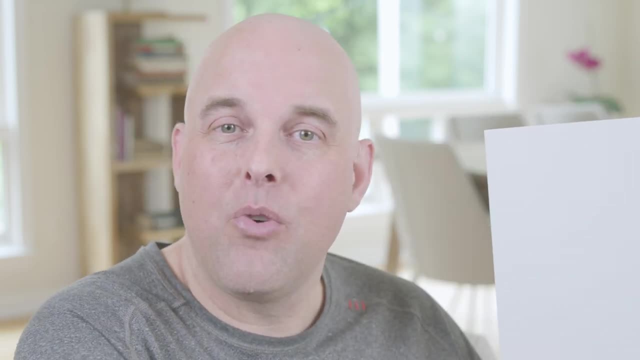 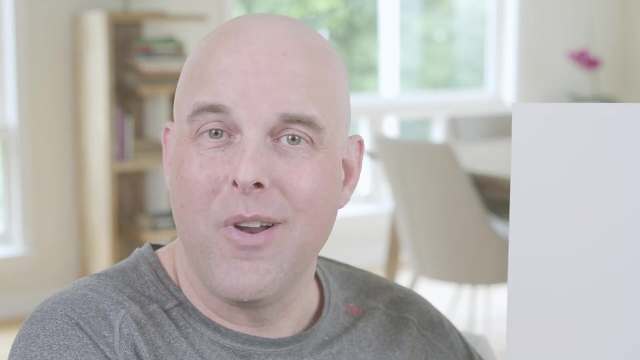 Gray by Benjamin Moore. It's a cool gray. It has a blue gray undertone, And watch what happens when I compare it with the warm gray that's called Revere Pewter by Benjamin Moore. Watch this, You're going to instantly see that when I compare Stonington Gray with Revere. 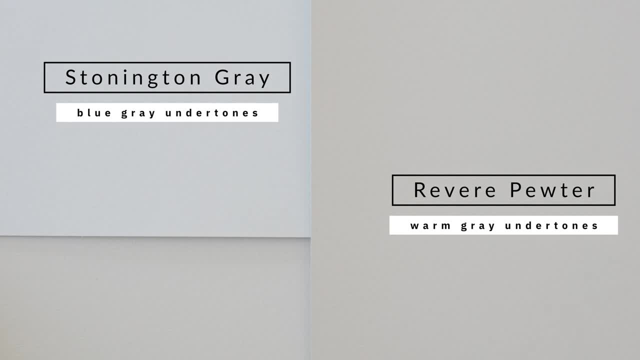 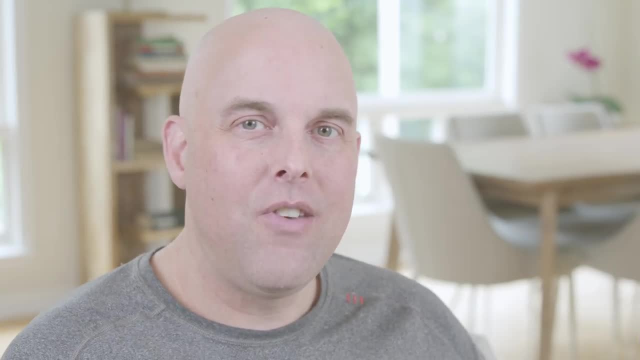 Pewter, you see that blue undertone in Stonington Gray. And then with Revere Pewter, you see that warm green. And then with Stonington Gray, you see that blue undertone in Stonington Gray. So there's a lot more to it than that. Now that you know that there's cool grays and warm grays, now 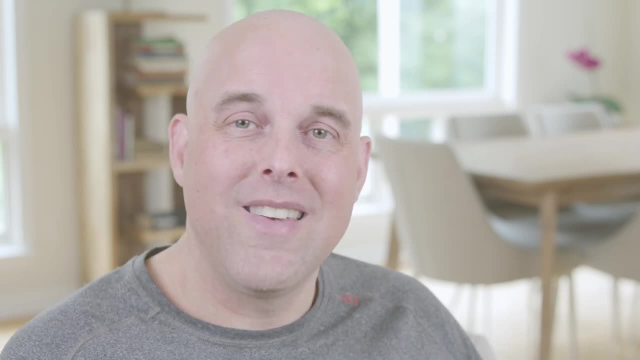 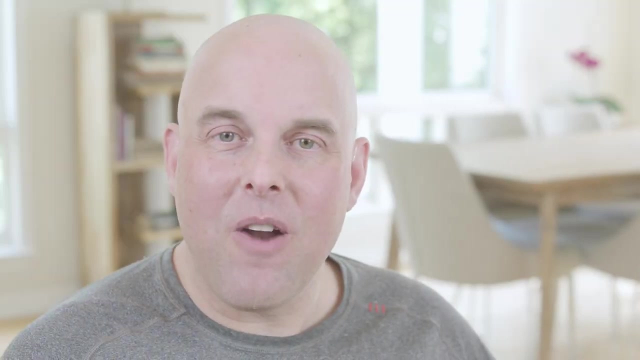 I want you to understand the different types of undertones of cool grays and warm grays, So next I'm going to show you the four different type of undertones that you need to know about. cool blue grays. Finding the perfect cool gray for your home is a lot more complicated than you may think. 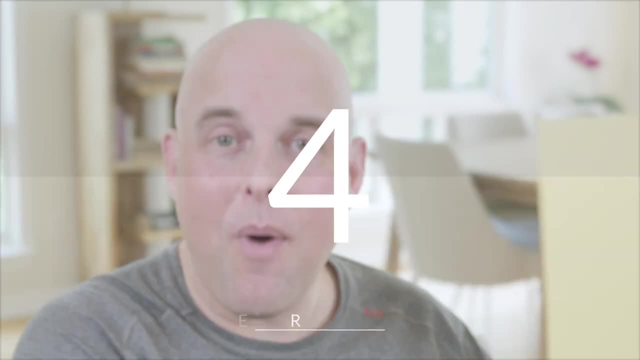 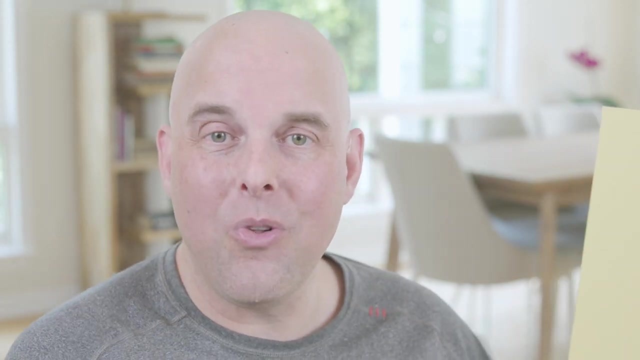 because there's four different undertones that you need to be aware of. I've selected Marblehead Gold by Benjamin Moore, which is considered a yellow. The reason why is because this yellow is going to pull out these different undertones that I'm about. 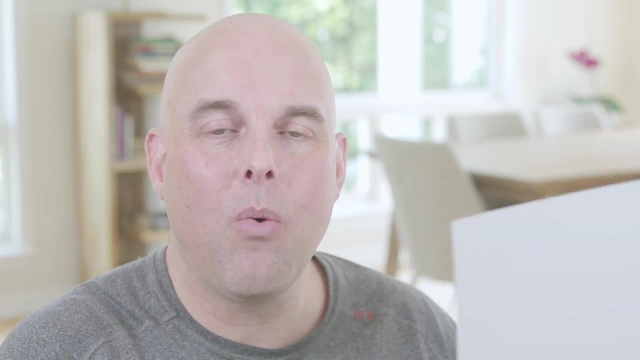 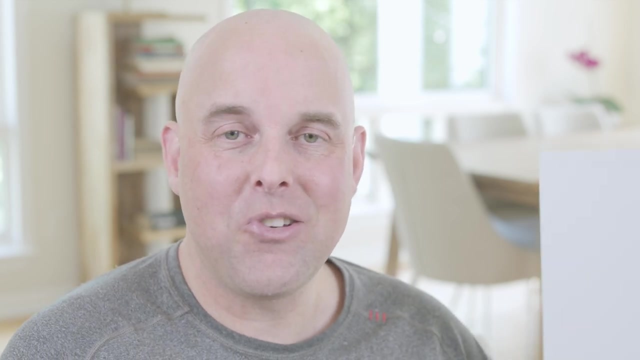 to show you. So watch this. The first undertone that you need to be aware of are blue grays, such as Sherwin-Williams Passive. There's a lot of popular blue grays out there, such as Stonington Gray, Coventry Gray or even Repose Gray, just to name a few. Watch what. 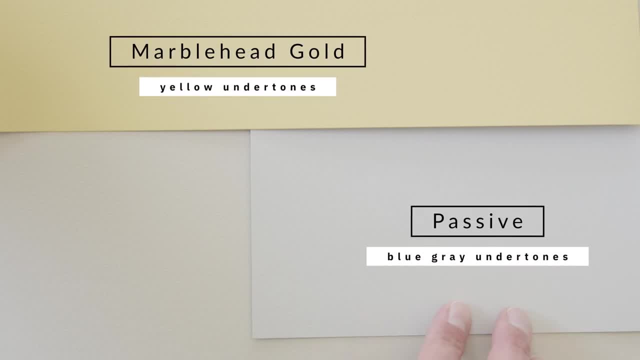 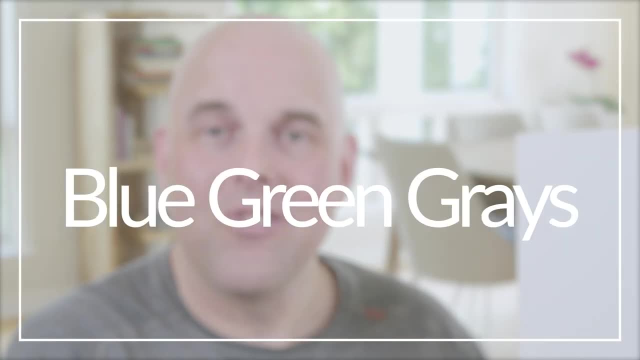 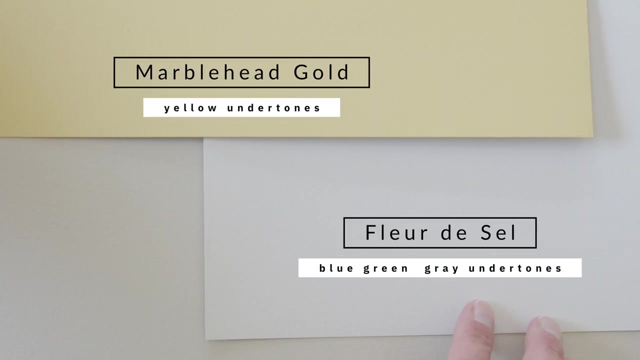 happens. when I compare Passive with Marblehead Gold, You're going to instantly see the blue gray. The next one that you need to be aware of are blue-green grays, such as Fleur de Sel. Watch this: When you compare Fleur de Sel, you're going to see that blue gray. and if 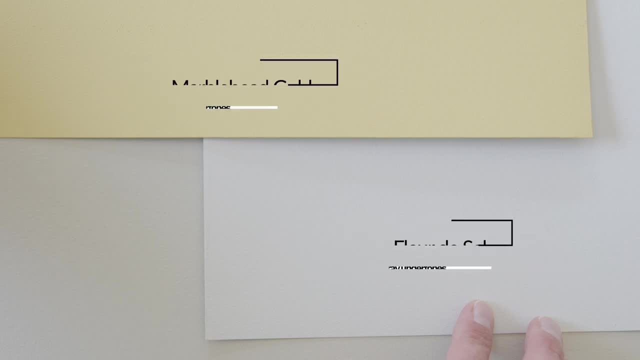 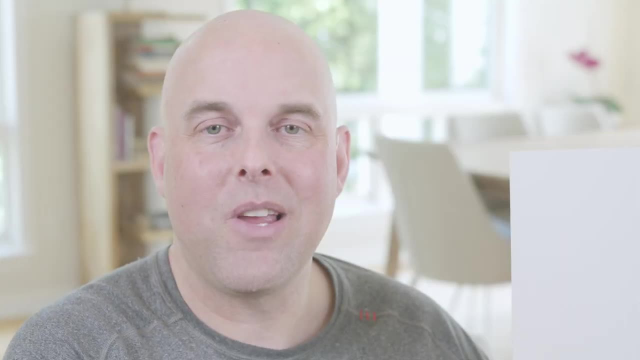 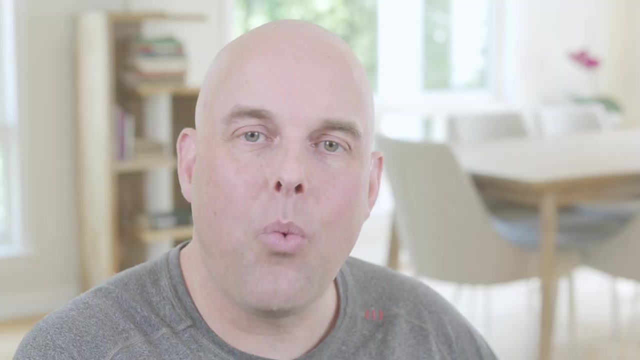 you look carefully, there's just a little bit of a green gray. The next one you need to be aware of are violet grays, such as Collingwood. Watch what happens when I compare Collingwood with Marblehead Gold. You're going to instantly see the violet gray. and there's one last. 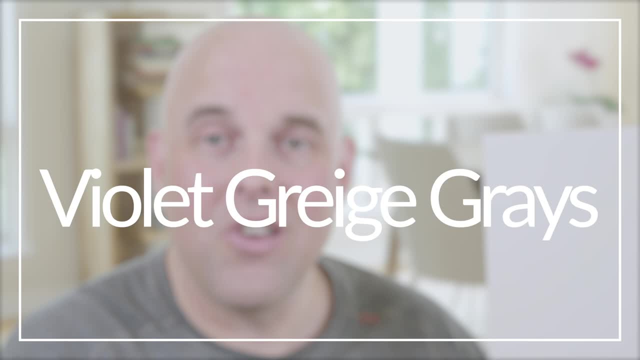 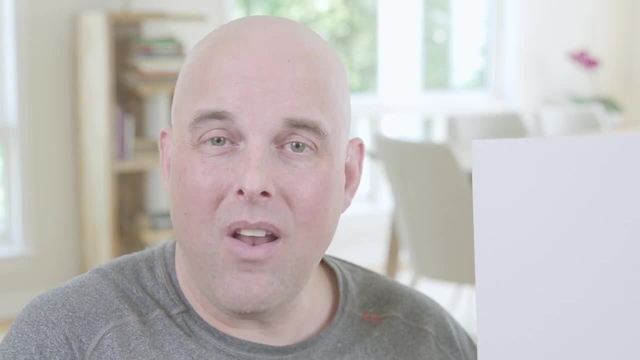 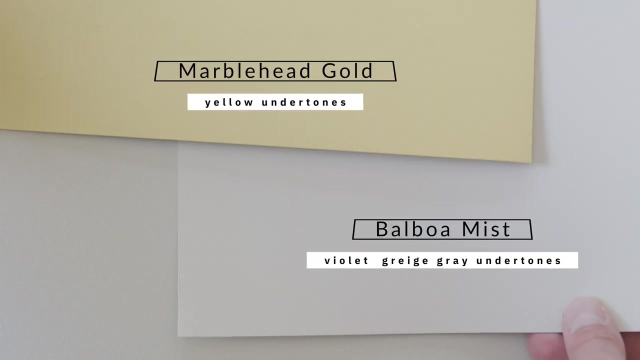 one that you need to be aware of: violet grays such as Balboa Mist. A violet gray means that a violet can actually be warm, but it also can lean on the cool side. Watch what happens when I compare Balboa Mist with Marblehead Gold. You're going to see the warmth of Balboa. 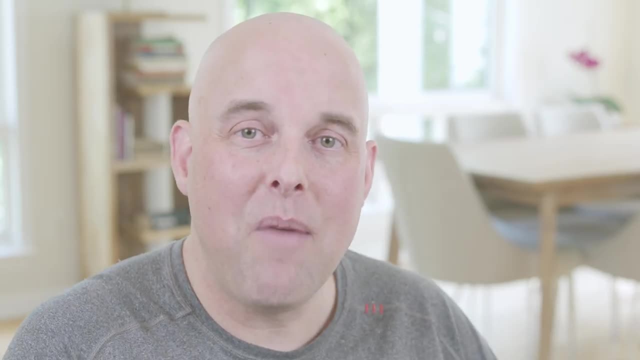 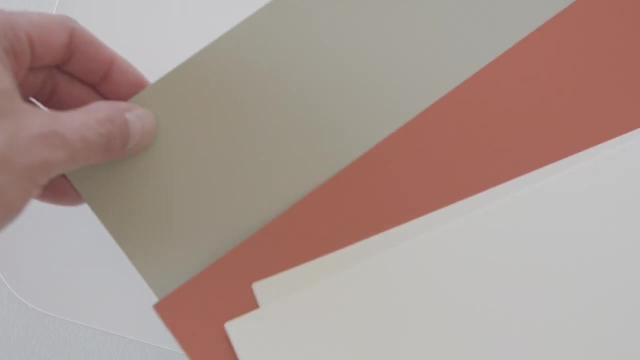 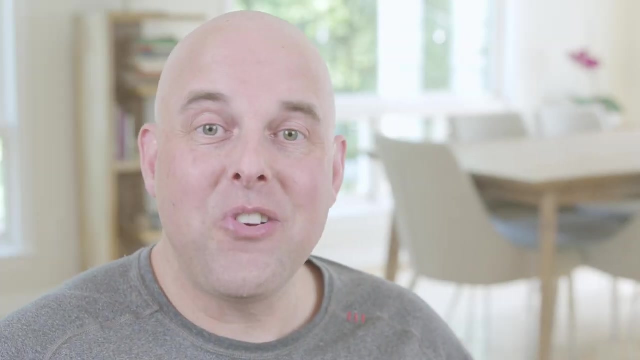 warm grey in the plum, firedus and some of the cool grays and, most importantly, the undertones. The next I want to talk about are the two undertones that you need to know about warm grays. She's ready When it comes to green grays. there's only two undertones that you need to. 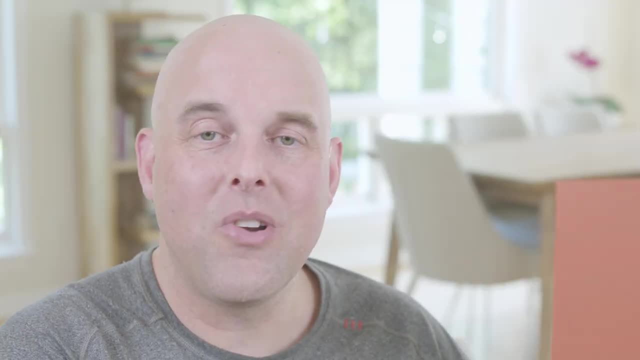 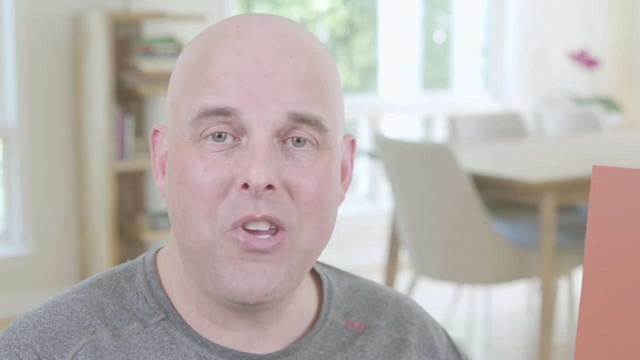 be aware of. So what I've done is I've selected Benjamin Moore'sSalsa Dancing. It's considered a red. It's a contrasting paint color. It's going to pull out these undertones that I want you to see. So the first undertone that you need to be aware of are green gray undertones. 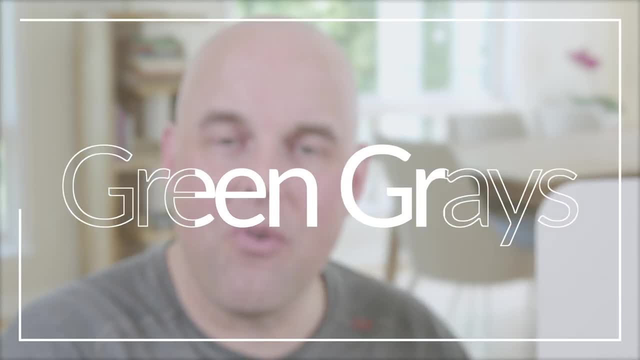 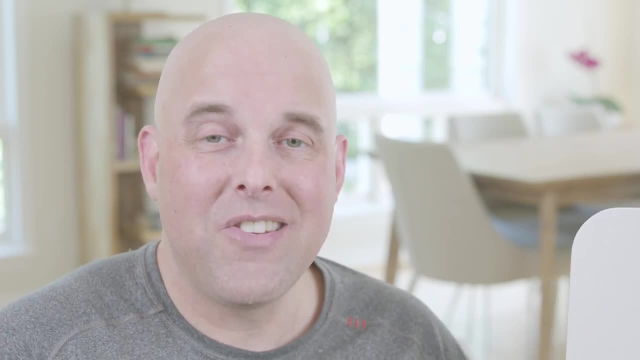 such as Macon Brown. That green is again the undertones that I want you to see, Green as Sherwin-Williams Modern Gray. Some other popular warm grays that you may be aware of are Edgecombe Gray, Revere Pewter, Accessible Beige, just to name a few. So watch what happens. 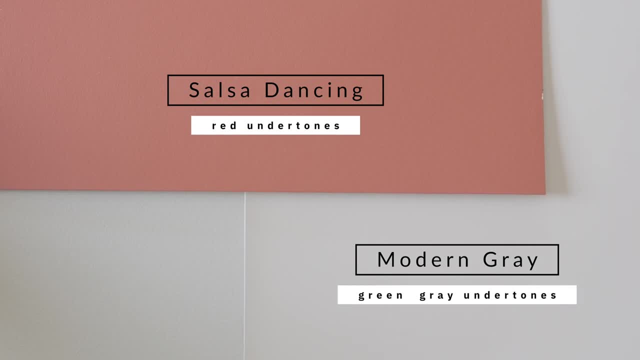 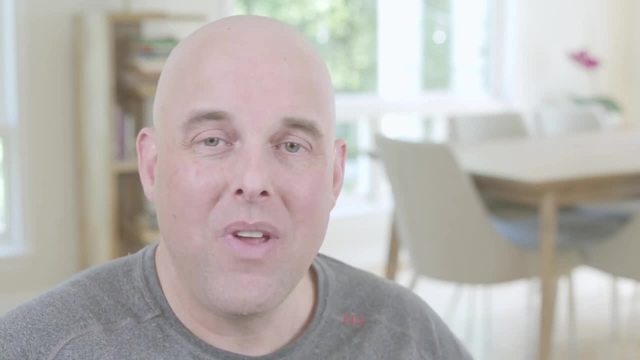 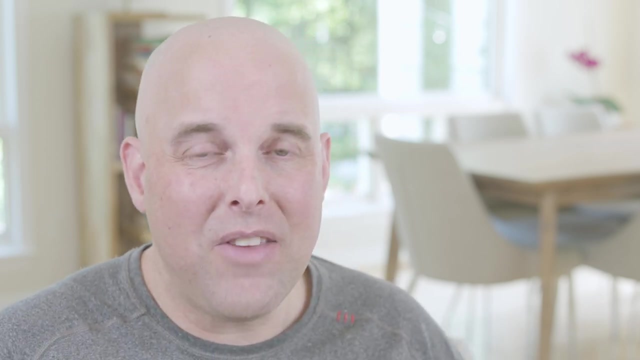 when I compare this with Salsa Dancing, You're going to instantly see the warm gray. Now be mindful: just because it's a warm gray and it has a green-gray undertone, it doesn't necessarily mean that your space will look green if you pair it correctly. So that's. 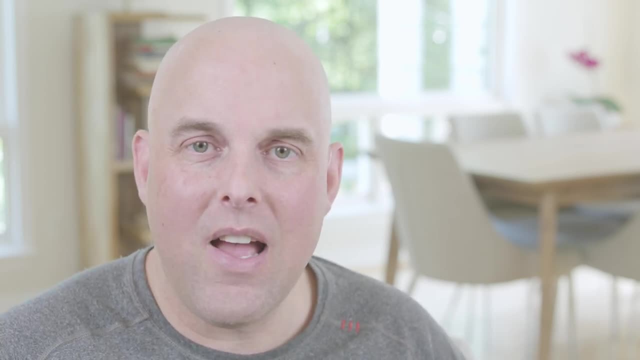 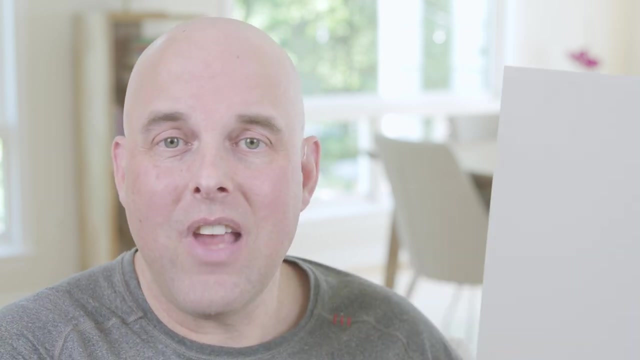 a lot more complicated and that's a different story for another time, But I wanted to show you another warm gray that's considered a green-gray, but it definitely will look green, such as Sandy Hook Gray. Watch what happens when I compare Sandy Hook Gray with Salsa. 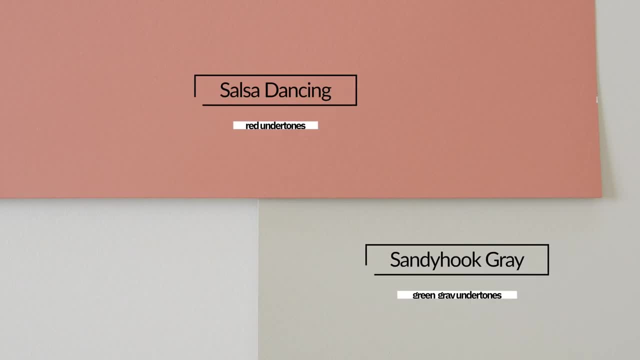 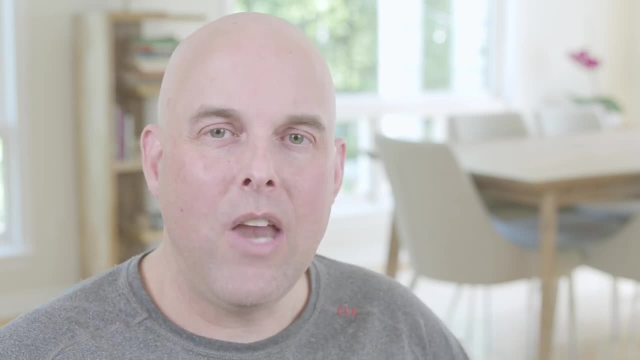 Dancing, You definitely see that green-gray undertone, So just be mindful when you're working with green-grays. Now there's another undertone that you need to be aware of, and you only find this on the very light spectrum of warm gray. 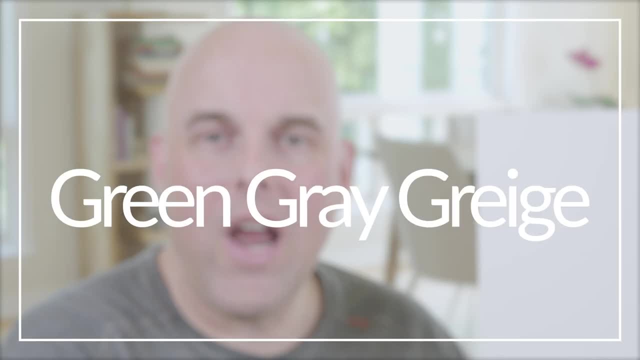 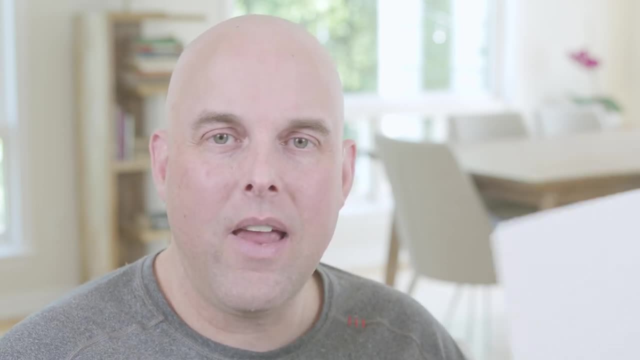 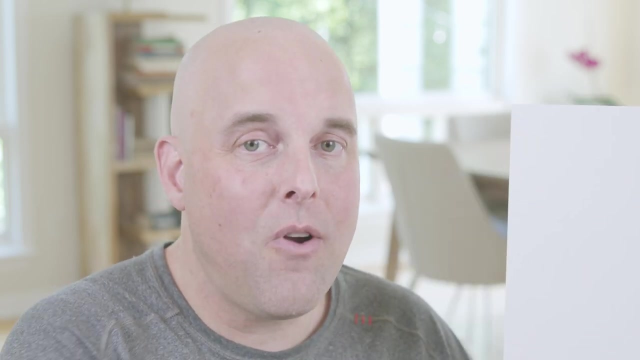 It's called Pearly White. It's a green-gray gray. This is the undertone that I want you to be mindful of. Now I want to show you an example of another light gray by Benjamin Moore, and it's called Classic Gray. Classic Gray is just a green-gray. Watch what happens. 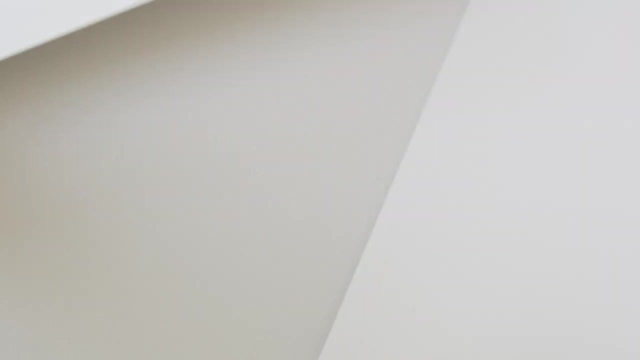 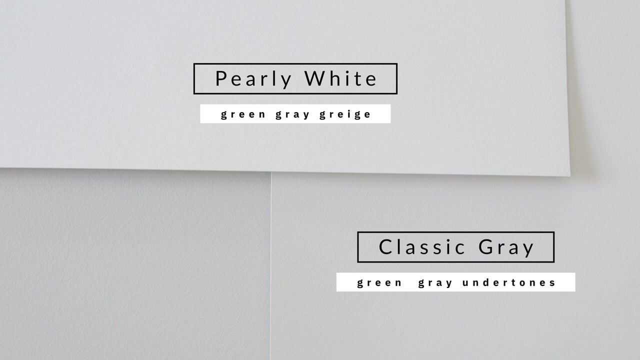 when I compare Classic Gray with Pearly White, When you compare Pearly White with Classic Gray, the first thing that you should notice is how Pearly White is very light. It's very light. It's warmer than Classic Gray. Classic Gray is cooler than Pearly White because 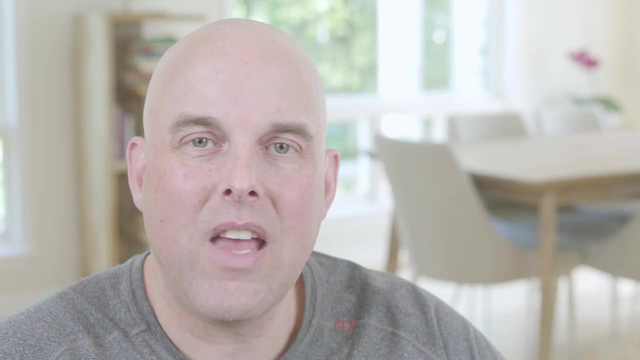 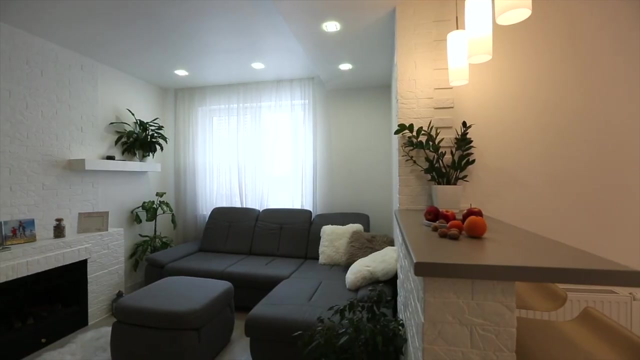 you're going to notice how Pearly White it just has more warmth because of that key word that I just said: grayish. It's got almost a little bit of a beige to it. So if you don't have a lot of natural lighting, for example, and you selected a super light, warm gray. 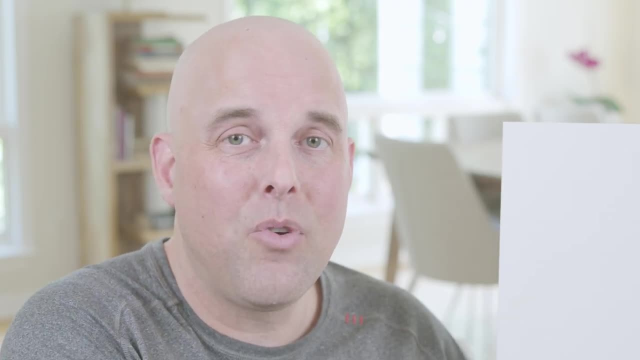 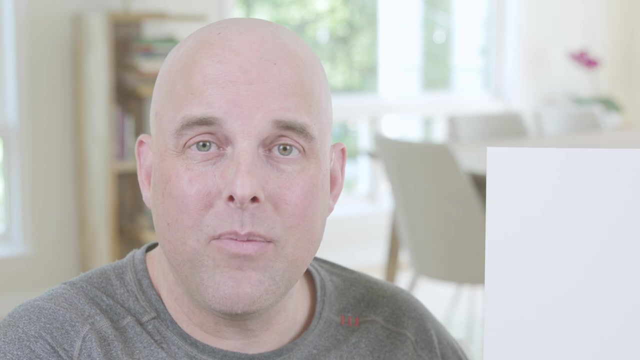 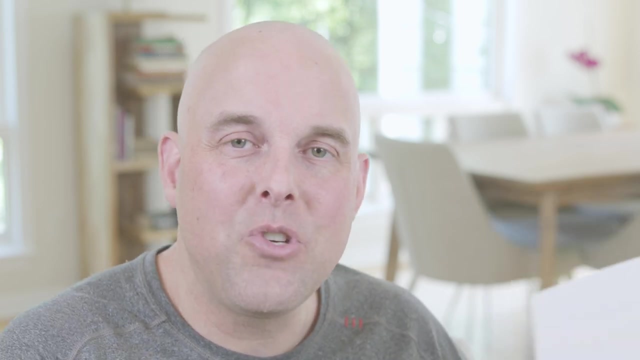 like Classic Gray. it could look like a blue-gray and it could look dingy. However, if you have Pearly White by Sherwin-Williams, you're going to get more warmth, not so much of that cool gray, especially if you don't have a lot of natural lighting. So those are two. 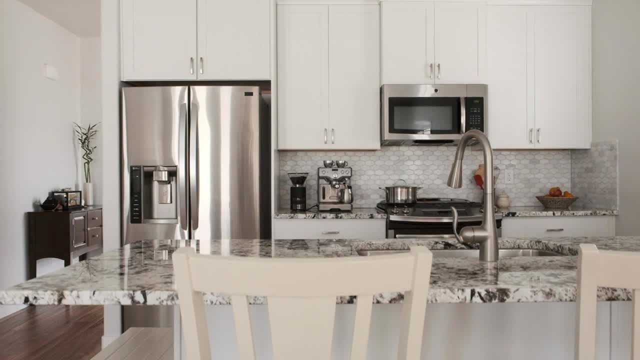 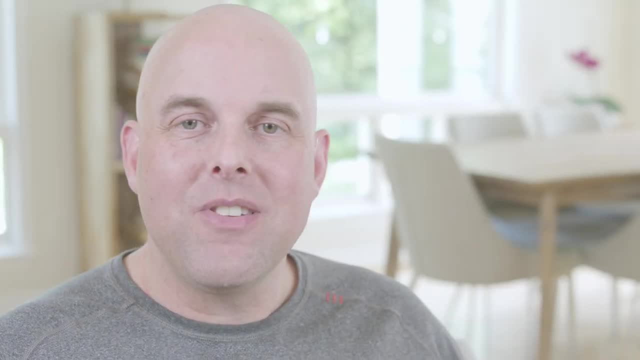 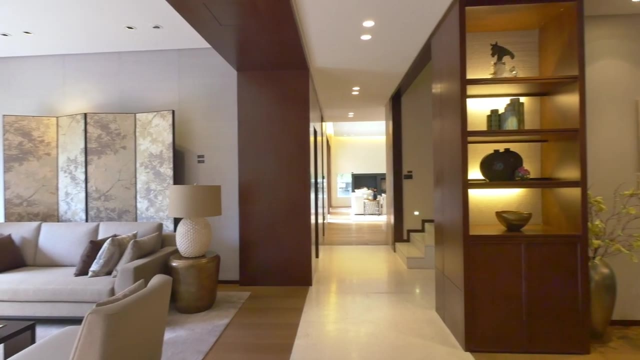 undertones that you need to know. And next I'm going to talk about the importance of comparing your gray paint colors with your fixed elements and lighting. One of the biggest mistakes that I see people make all the time is not pairing the correct paint color with their fixed elements and not being mindful of the type of natural and 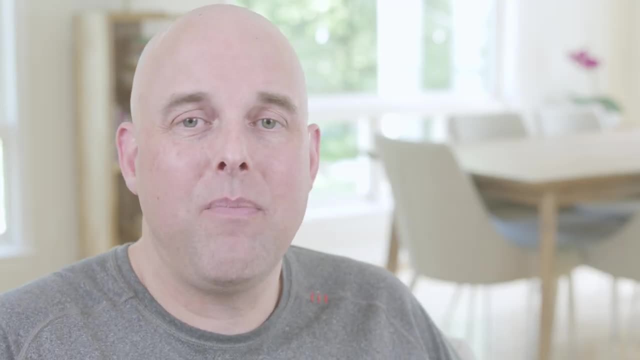 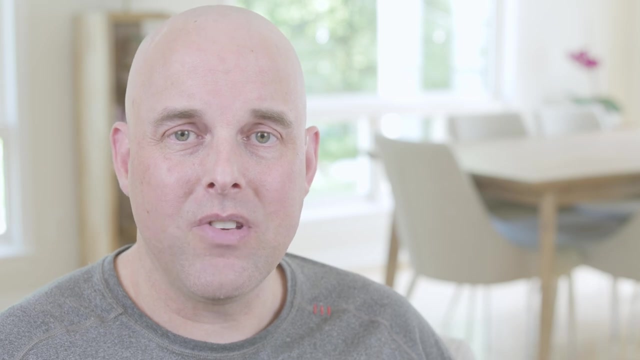 artificial lighting that they have in their home, and I don't want this to be you. You've got to get this right, especially when you're working with gray paint colors, because gray paint colors are chameleons, and that's an important word, right there: chameleon Undertones. 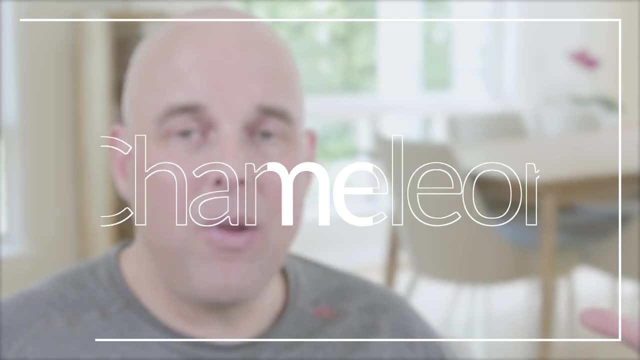 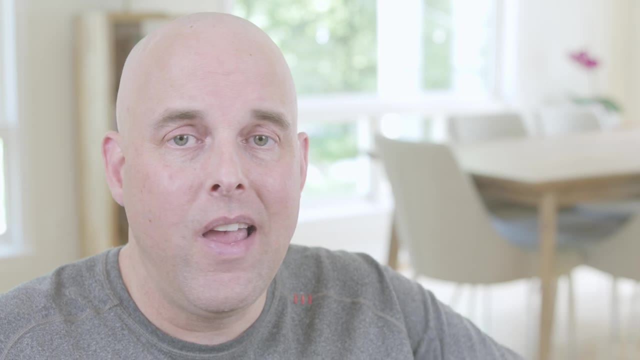 and grays are chameleons, and this is where you've got to be really mindful. if you're working with a cool gray or warm grays, Is it going to be a green-gray, Is it going to be a blue-gray, Is it going to be a blue-green-gray? 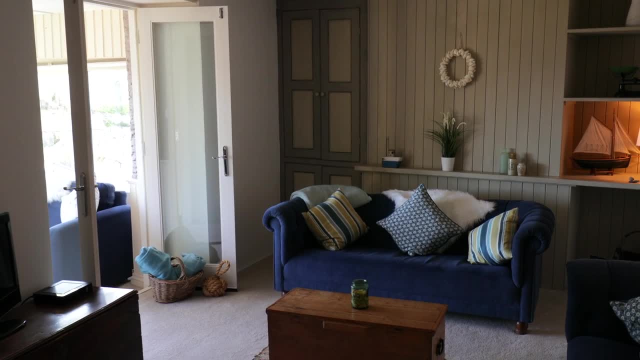 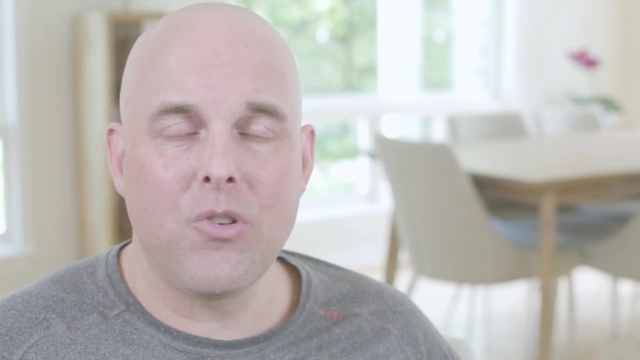 And you need to be mindful of the type of lighting that you receive in your home. So if you don't receive a lot of natural lighting, even if it's a north-facing, east-south or west, it doesn't matter If it's cool or warm, especially on the light spectrum of cool grays. 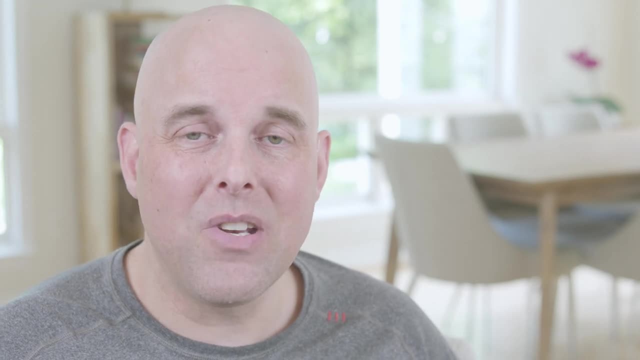 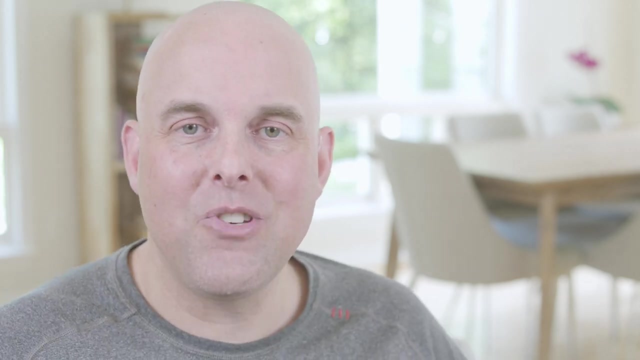 and warm grays. chances are your space is going to look dingy, It's going to look muted, So you need to be mindful of that. Also, when it comes to fixed elements, what type of fixed elements do you have If you're thinking about a cool gray in your space and you have beige? 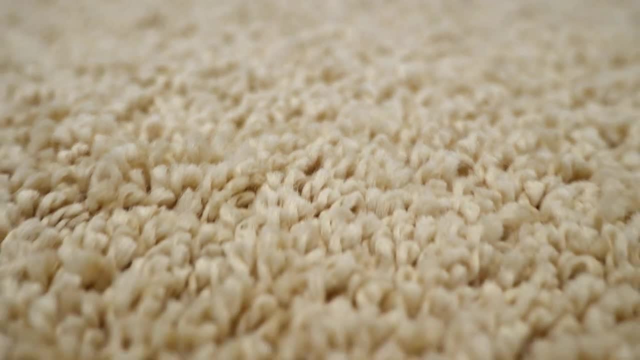 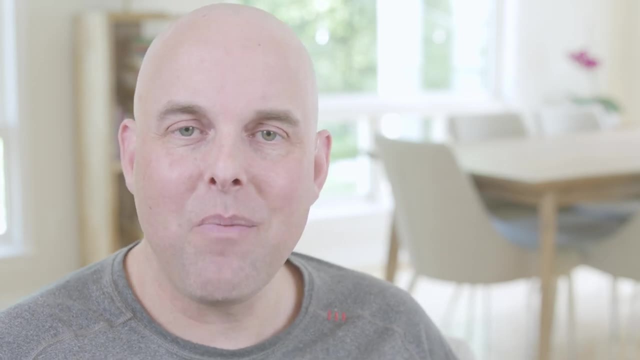 carpets, then chances are it's going to clash with your beige carpets because it's going to make them look old and dingy. You're going to get that blue-gray in it. It's too clean. Your carpet, your beige carpet, is muted, So it's dirty in comparison to that clean. 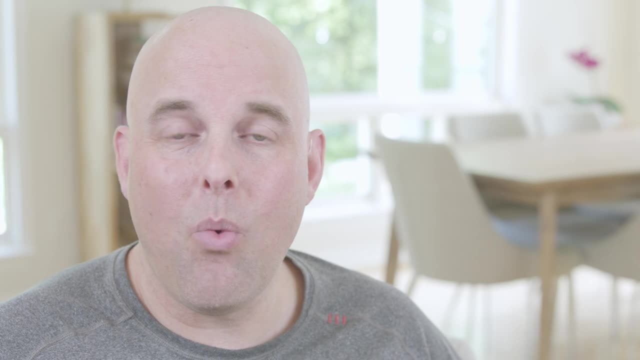 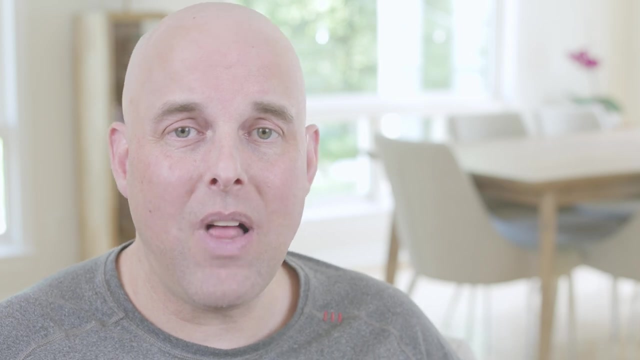 blue-gray. Perhaps you might want to compare it with a warm gray, but you've got to be careful because if it's classic gray it may not work. It might be too light. You might need to do something a little bit warmer, maybe light gray mist, for example. If you're 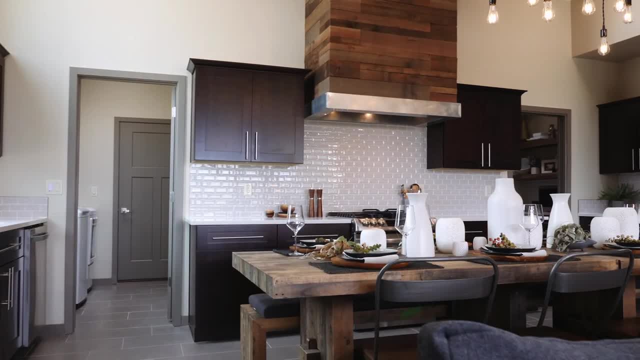 thinking about a cool gray in your space, then chances are it's going to clash with your beige carpet because it's too light. You might need to do something a little bit warmer, maybe light gray mist, for example. So you need to be mindful of the type of lighting.